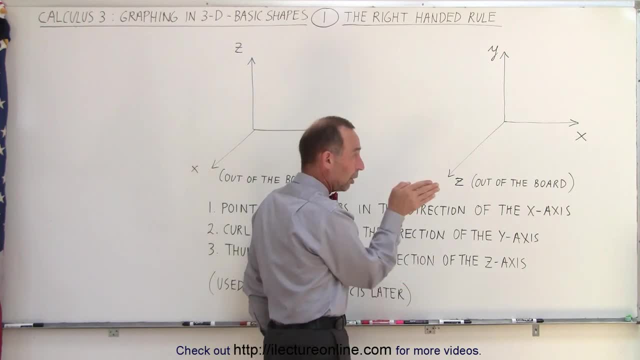 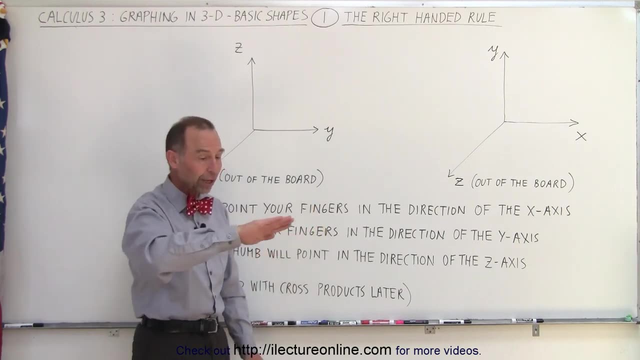 fingers in the direction of the x-axis. so we'll go ahead and do that over here: point in the direction of the x-axis and the next thing we want to do is curl your fingers in the direction of the y-axis. well, in order to do that, you may. 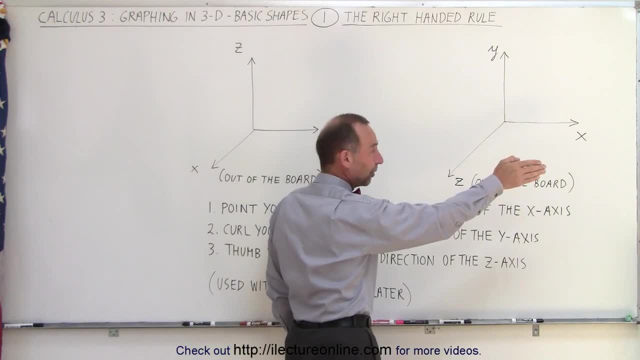 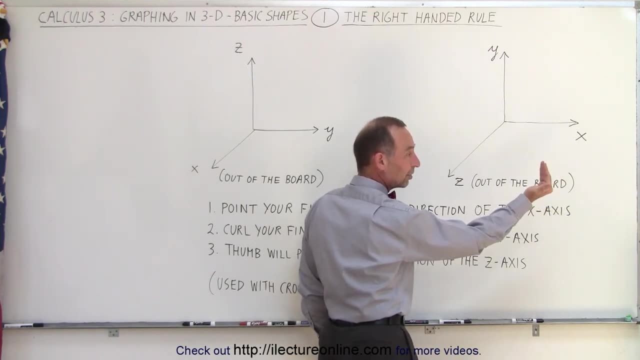 have to turn your hand around to make that happen. so here we need to turn our hand this way, and now we're going to curl fingers in the y-direction, so we point in the x-direction, then we curl our fingers in the y-direction and then, if we stick out our thumb, our thumb will point in the direction of the z-axis. so 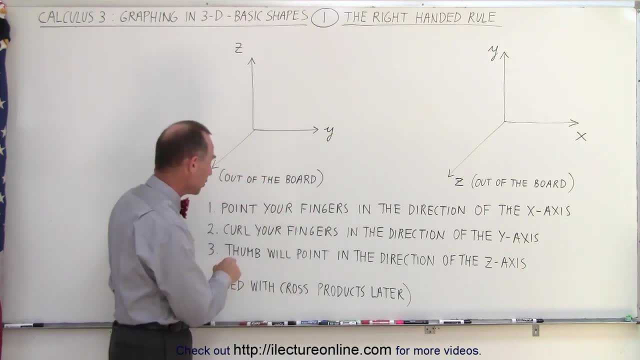 that X, Y, Z, and that's exactly what we'll do here. point your fingers in the direction of the x-axis, curl your fingers in the direction of the y-axis, and your thumb will point in the direction of the z-axis. now, if these two are the same, we should 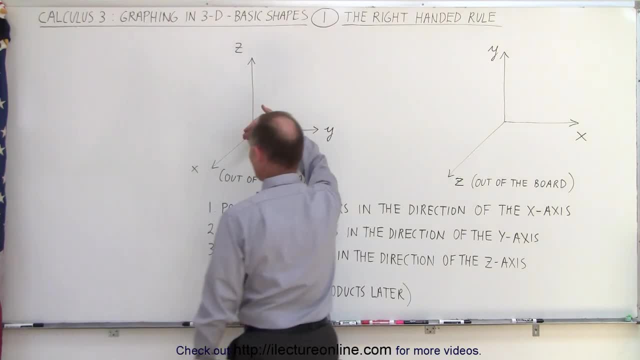 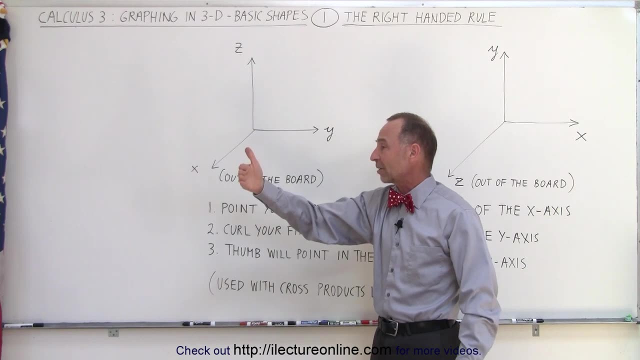 get the exact same result. so let's see here we need to point our fingers in the direction of the x-axis, which is out of the board. then we want to curl our fingers in the direction of the y-axis. that means I have to have my hand like 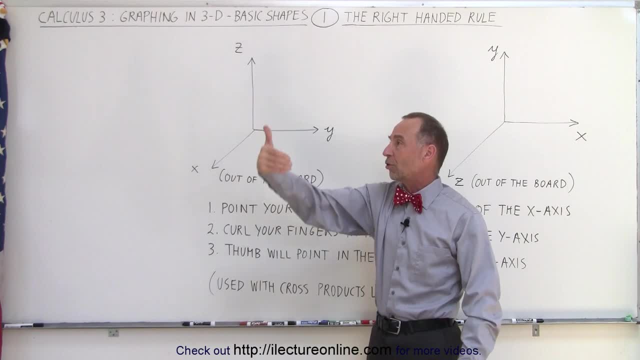 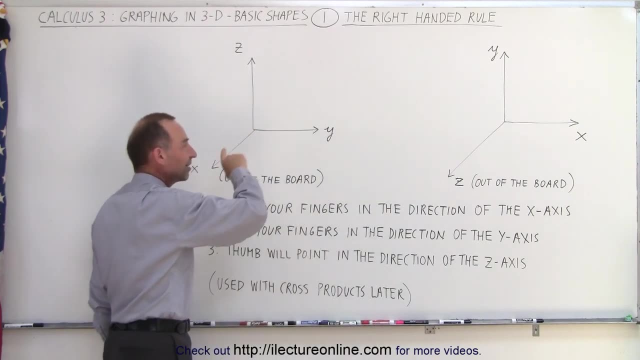 this: so x-axis, curl fingers in the y-axis and the thumb will point in the z-direction, which is straight up. so there you can see that, using the right hand rule, those are the exact same representation of three-dimensional space and that's how we can check it out, and using that right hand rule. 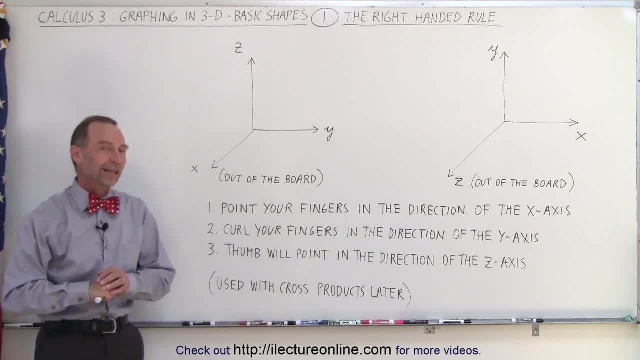 will come in very handy when we're dealing with cross products of vectors later in three-dimensional space. so there's our start and we'll have all kinds of other good nuggets, so to speak, good piece of understanding in three-dimensional space before we move on to using vectors in three-dimensional. 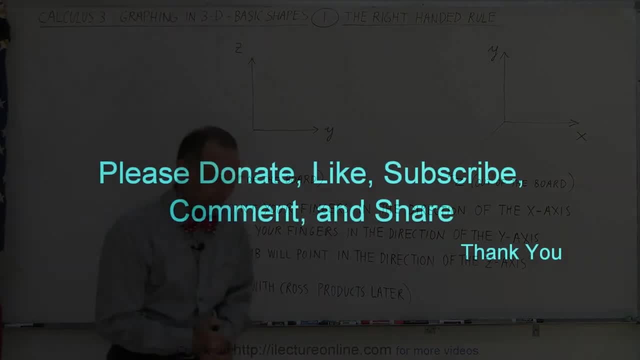 space. that's how it's done. 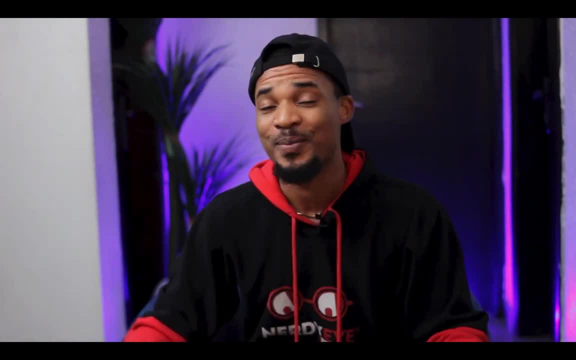 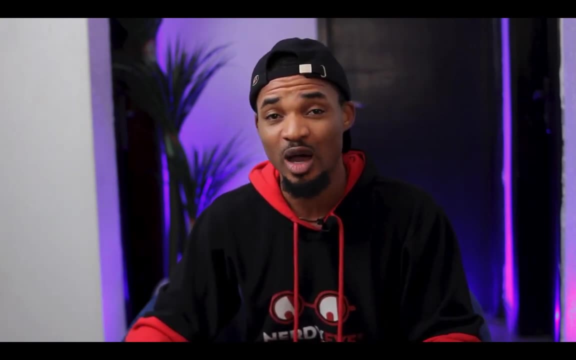 Hi guys, thank you so much for joining this seven days class. My name is Samon Linus and I'm super excited to have you here. At Nerdy Eye. we're a peer-to-peer edtech platform that allows people to learn in peers, groups and communities. It simply means that gone are those days when you